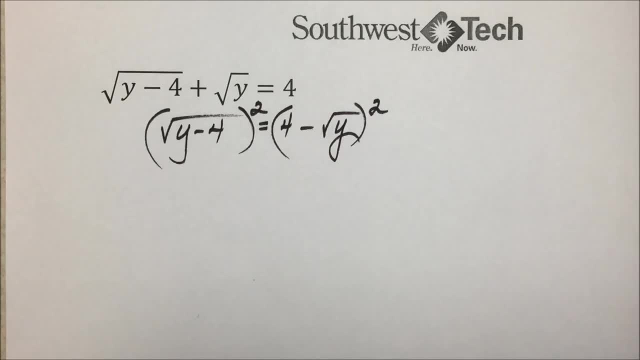 going to get rid of all of our radicals in one Step, like we do when we have an equation with just one radical Here. when we raise a- in this case a square root- to the second power, we get the radicand On the right-hand. 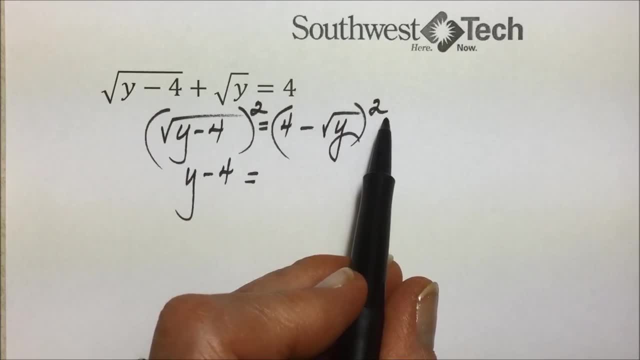 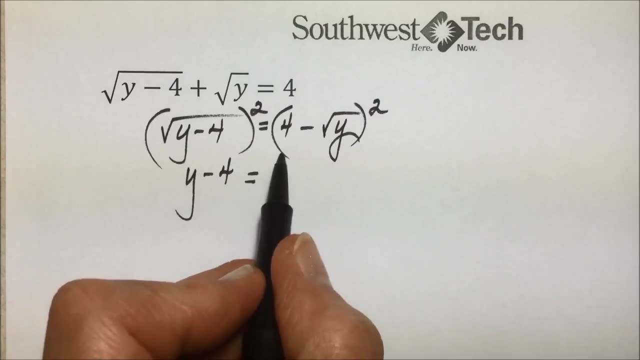 side we have a binomial raised to the second power. If you know the shortcut, we can square the first term, square the second term, multiply the two together and double them. Otherwise this is the equivalent of 4 minus square root of y. 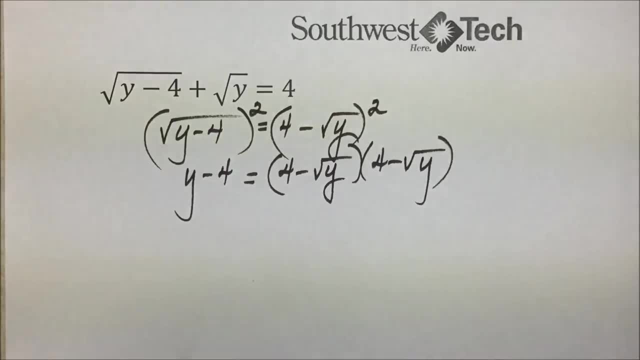 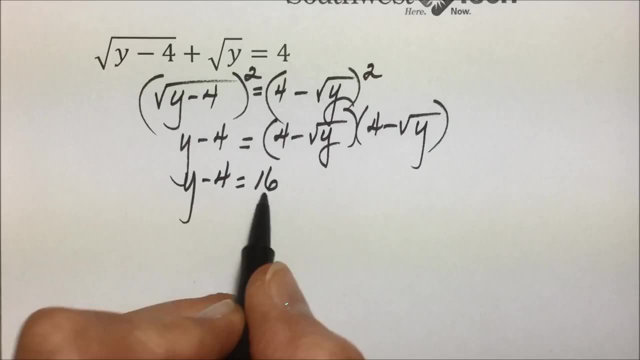 Step, like we do when we have an equation with just one radical Here, when we raise a, in this case a square root of y times 4 minus square root of y, where we will use FOIL method to simplify. So we have a y minus 4.. First terms multiplied together is 16.. 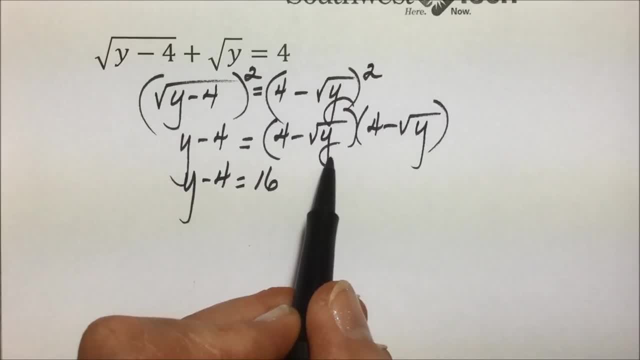 Outside would be a negative 4 times the square root of y. Inside terms would be another negative, 4 times the square root of y, which makes a negative 8 times the square root of y. Last terms multiplied together. a negative times a negative is positive. Square root of y times. 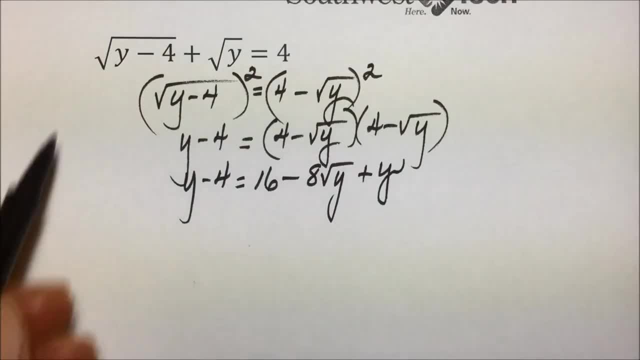 square root of y is y. Well, we started with two radicals, We're down to one. Let's isolate it. And first things first, how about subtracting a y from each side? and while I'm at it, I'm going to subtract. 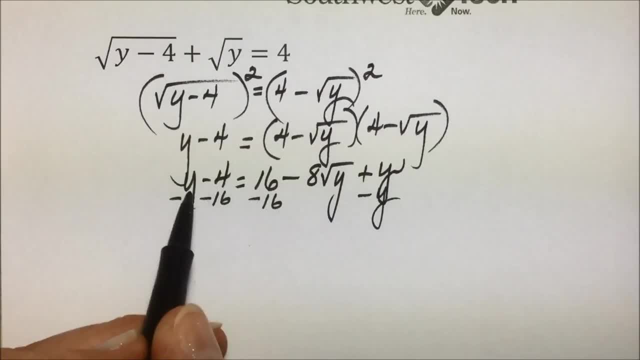 a 16 from each side. The y's are gone. Negative 4 minus 16, or plus a negative 16, leaves us with a negative 20.. Sixteens are gone: Equal to a negative 8 times the square root. 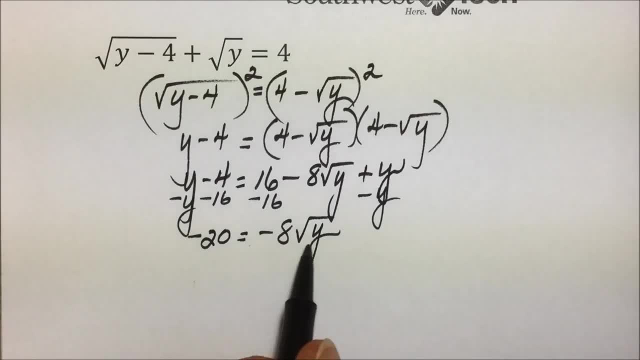 of y. We could square both sides at this point, but we don't want to do that, So we're going to subtract the y from each side And, while I'm at it, I'm going to subtract a 16 from each side. And while I'm at it, I'm going to subtract a 16 from each side. So we're going to subtract a 16 from each side And while I'm at it, I'm going to subtract a 16 from each side. 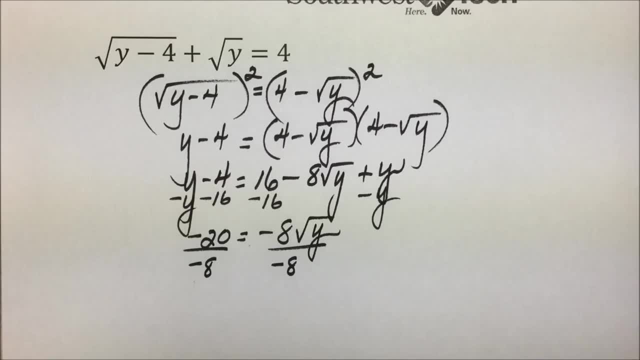 I'm going to subtract a 16 from each side. Now let's get into the basically the negative part, and that's just to make it easier. Then I divide both sides by eight, so that the radical truly is by itself The negatives. 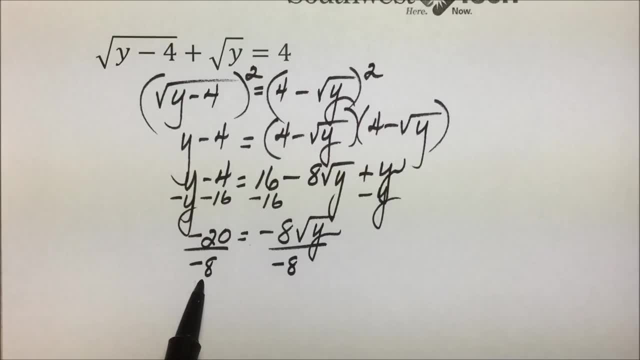 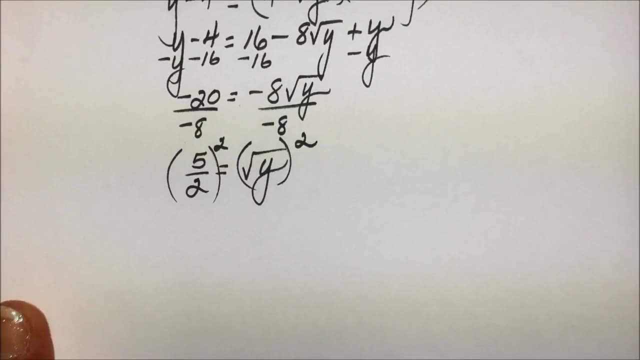 cancel out. Twenty-eighths has a common 4, leaving us with 5 halves is equal to the square root of y. Now ready to raise each side to the second power to eliminate this last radical Five halves. squared times 5 halves is 25 fourths. A radical squared is the radicand and I believe that's the. 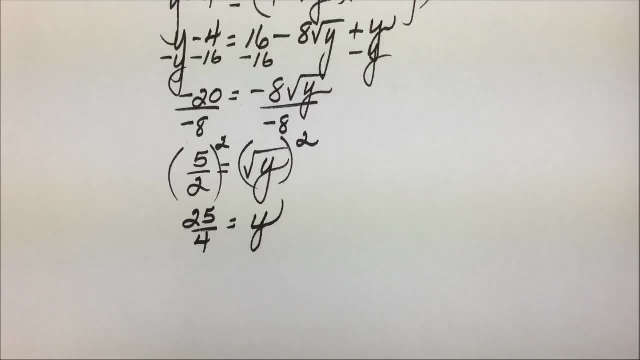 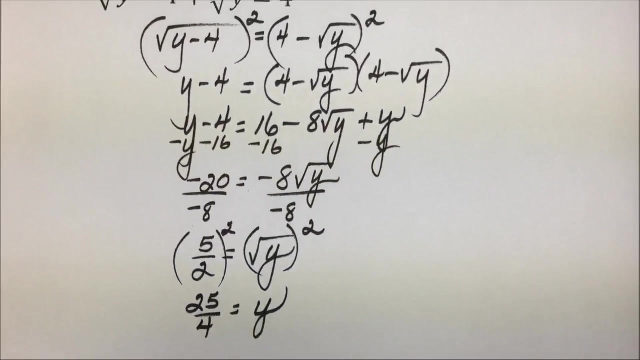 solution is 25 fourths. Because the principle of powers is not always true. it's always essential that you plug that solution or solutions into your original equation, and if there's a chance of ever generating a false solution, it's when you are squaring, or whatever the 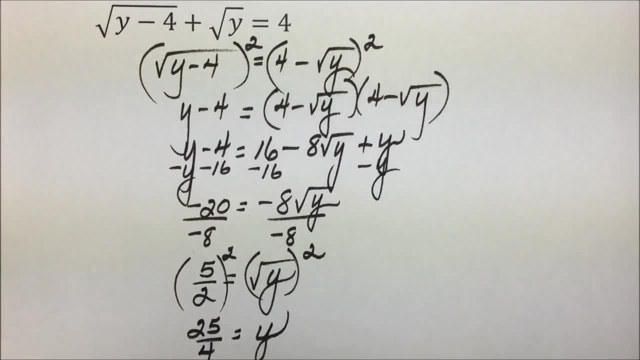 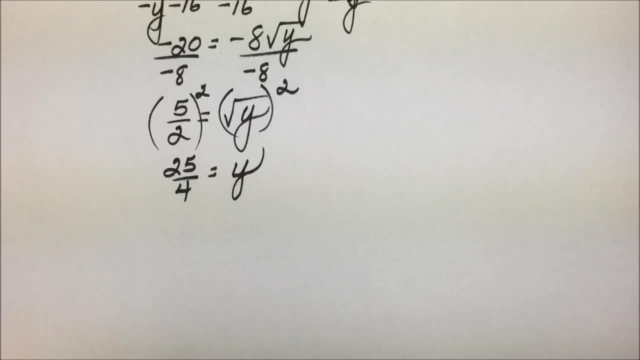 power is you're raising both sides to more than once, Chances are you can generate an extraneous root at that time. So just to show the check here, it will be the square root of y, which is 25 fourths minus 4, plus the square root of y, which is 25 fourths minus. 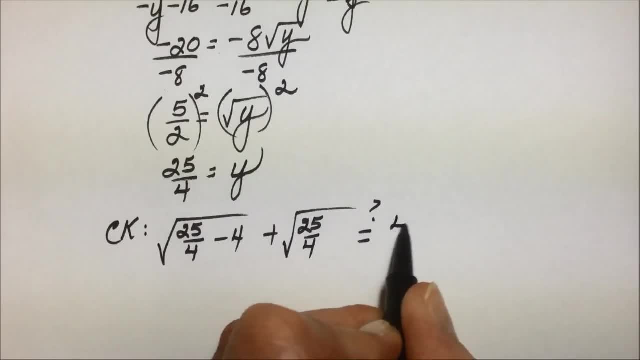 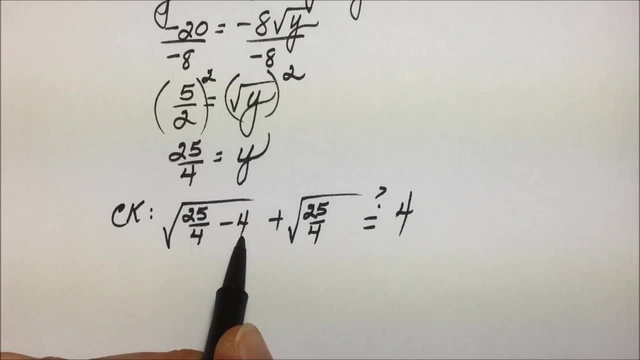 the square root of y, which is 25 fourths minus 4, plus the square root of y, which we found to be 25 fourths, and we're looking to see if that is equal to 4.. To simplify, underneath the radical, we need a common denominator. 4 is a denominator of 1, so we'll multiply. 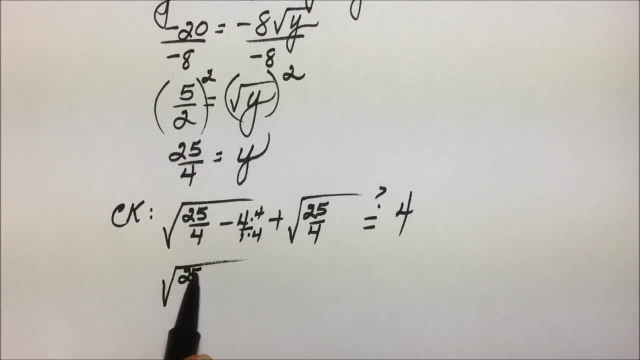 top and bottom by 4.. That will give us 25 fourths minus 16 fourths. Square root of 25 fourths is 5 halves. Simplifying further: 25 minus 16 is 9 fourths. So we're going to. 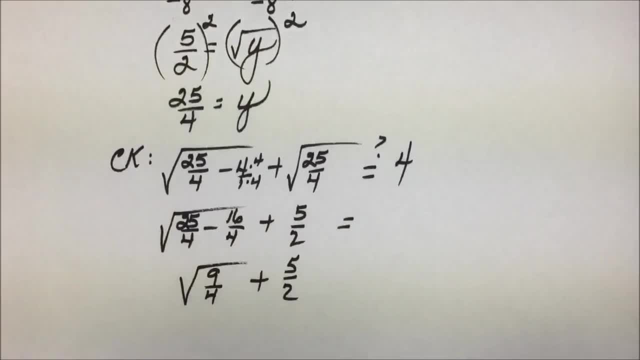 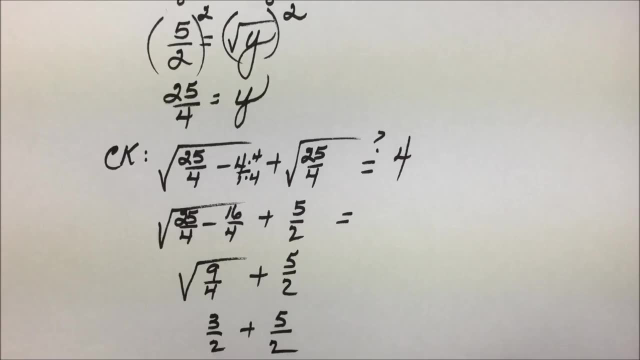 get 9 fourths. Square root of 9 is 3.. Square root of 4 is 2.. 3 halves plus 5 halves is 8 halves, which equals the 4 that we were looking for. So it does turn out that 25 fourths. 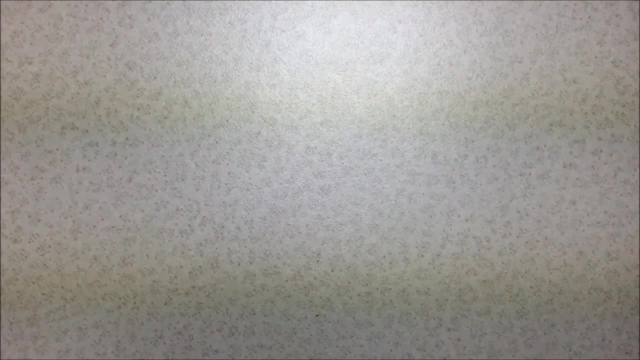 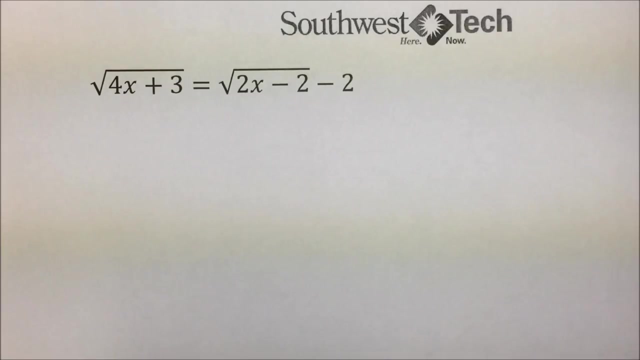 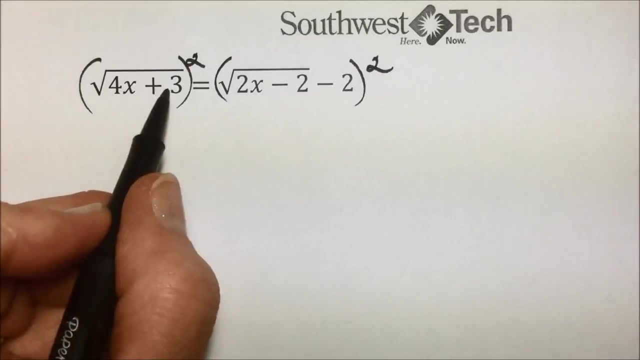 is our solution to this radical equation. Let's look at another one. Here we have our two radicals, and the procedure is to isolate the radical term on one side of the equation. It's already done so we're set up and ready to go. We're going to square both sides of the equation. Squaring a radical gives us. 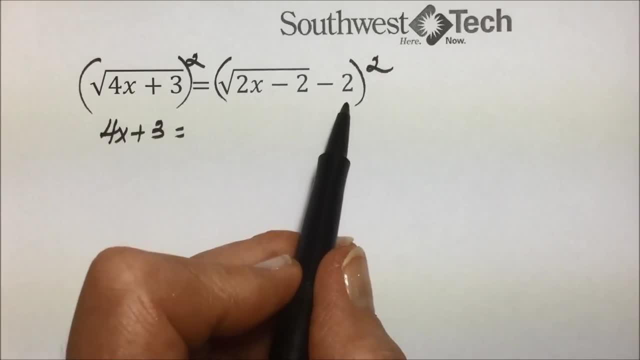 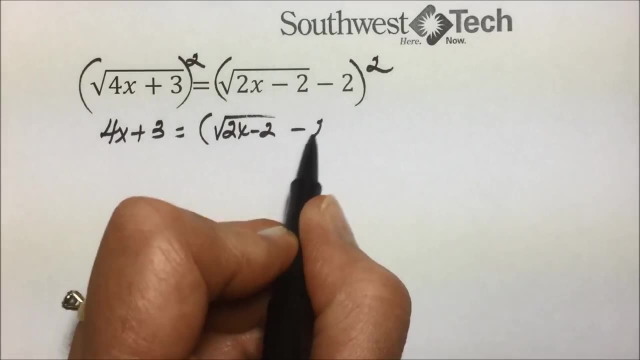 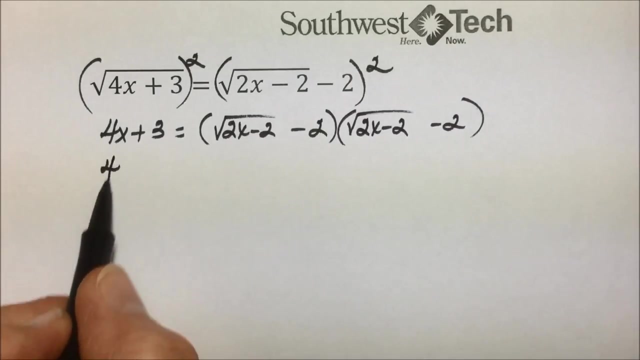 the radicand, And just like the last one, we have a binomial here- times itself. So we have the square root of 2x minus 2 minus 2 times the square root of 2x minus 2 minus 2, where we'll use the FOIL method to simplify this, Multiplying the first two terms together: 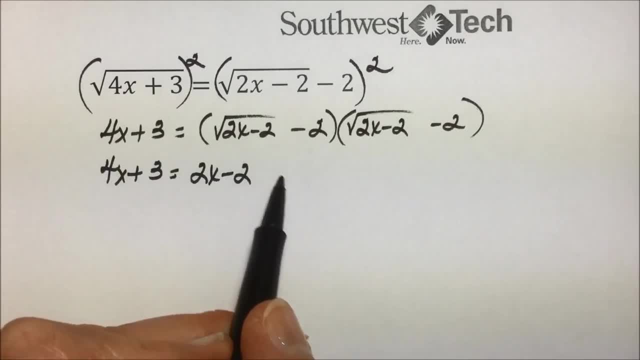 gives us the radicand of 2x minus 2.. Outside we'd have a negative 2 times the radical. Inside we'd have another negative 2 times the radical. Negative 2 and negative 2 makes a negative 4.. 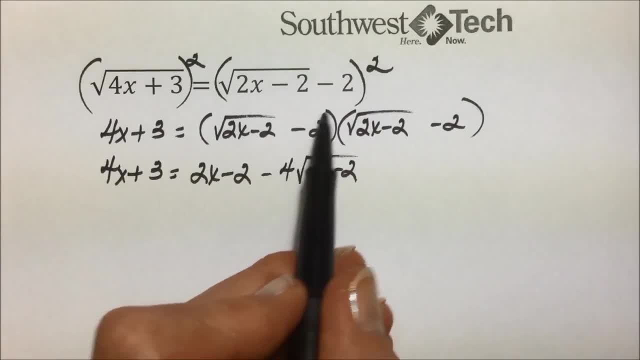 So we'll use negative 2 times the square root of the radical And the last terms multiplied together: a negative times a negative is a positive. 2 times 2 is 4.. So, good news, we eliminated one of the two radicals with that procedure. Next we'll want to get our terms. 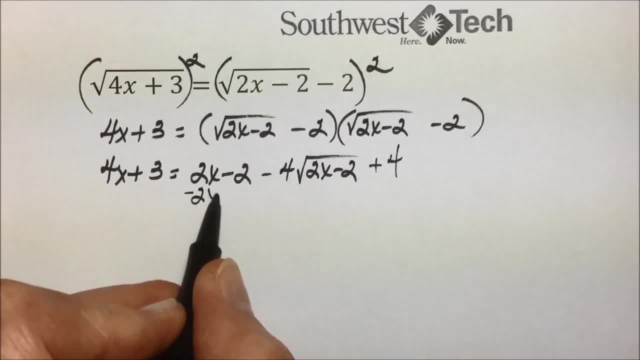 together, I'm going to subtract a 2x from each side. 4x minus 2x leaves us with a 2x plus 3.. out we have a negative 2 plus 4. now these are on the same side, which gives. 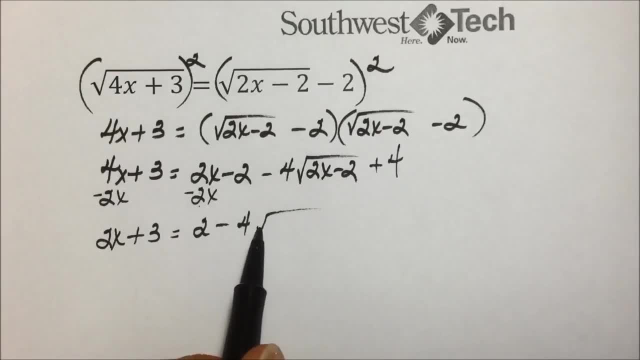 us a 2 minus 4 times the square root of our 2x minus 2. to get this last radical by itself is our next goal. so continuing to pull off common values. subtracting a 2 from each side leaves a 2x plus 1 on the left. the twos are gone. a negative.